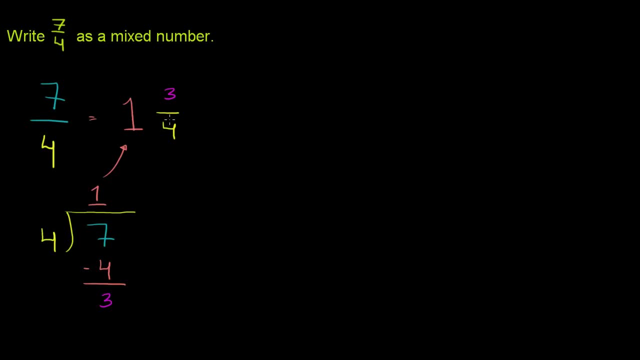 And maybe it'll become clear. So let's do a little square as a fourth. So I'm going to do it. Let's say I have a square like that And that is 1 fourth. Now let's think about what 7 of those mean. 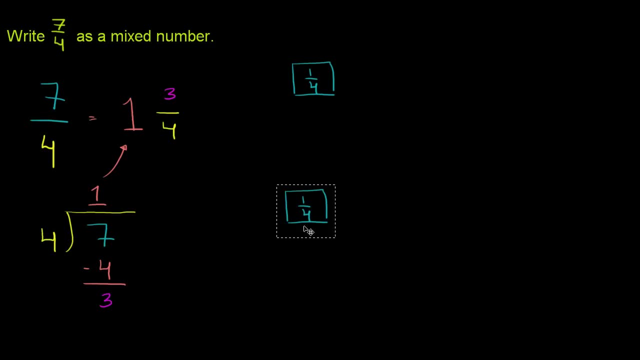 So let me copy and paste that Copy and then paste it. So here I have 2, 1 fourths. Or you could say: I have 2 fourths, Now I have 3, 1 fourths, Now I have 4, 1 fourths. 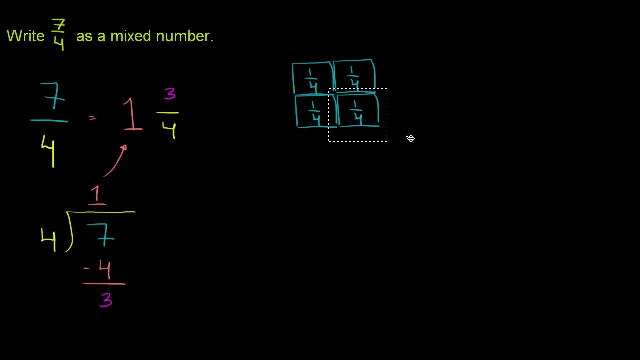 Now this is a whole right. I have 4: 1 fourths. This is a whole, So let me start on another whole. So now I have 5.. Now I have 6: 1 fourths, And now I have 7: 1 fourths. 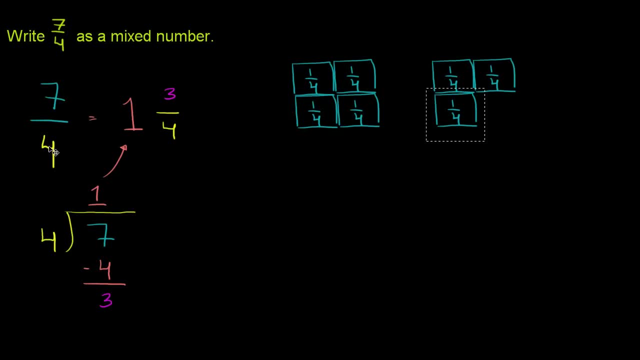 Now what does this look like? So all I did is I rewrote 7 fourths, or 7: 1 fourths. I just kind of drew it for you. Now what does this represent? Well, I have 4 fourths here. 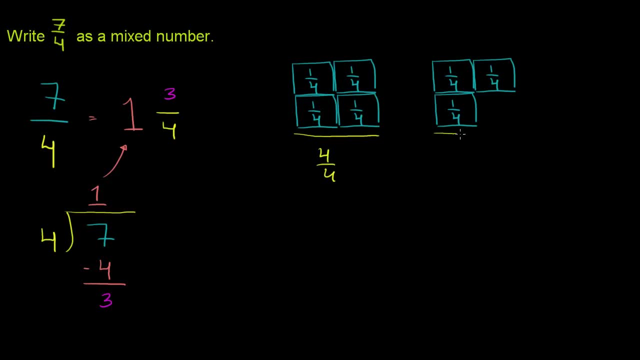 So this is 4 over 4.. This right here is 3 over 4.. Notice: 7 over 4 is 4 fourths, with 3 fourths left over. So let me write it this way: 7 over 4 is 4 fourths, with 3 fourths left over. 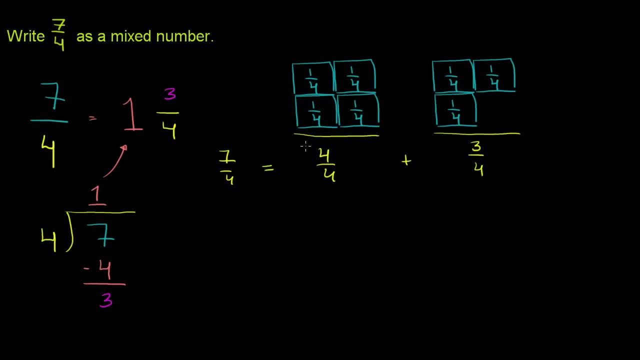 Now, what is 4 fourths? What is 4 fourths? 4 fourths is 1 whole, So you have 1 whole with 3 fourths left over. So you end up with 1 and 3 fourths. 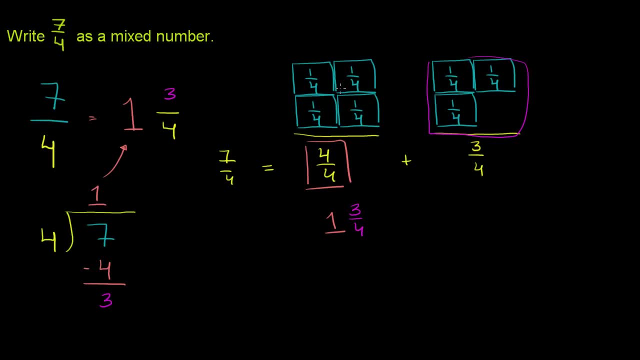 So that is the 3 fourths part And that is your 1 whole. Hopefully that makes sense And hopefully you understand why it connects, Because you say: well, how many wholes do you have When you're dividing the 4 into the 7 and getting the 1,? 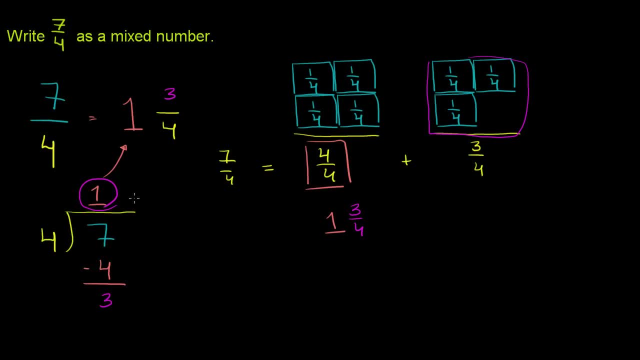 you're essentially saying how many wholes, So the number of wholes, Or you can imagine the number of whole pies. And then how many pieces do we have left over? Well, we have 3 pieces And each piece is a fourth. 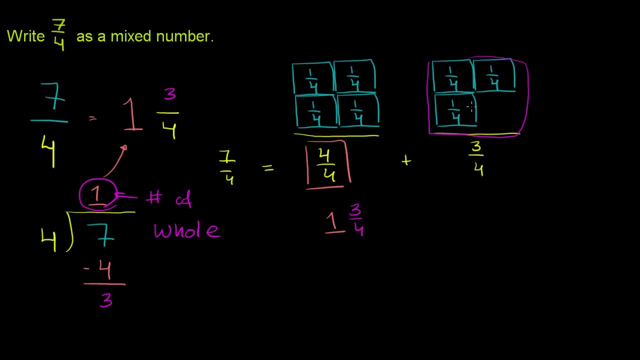 So we have 3 fourths left over. So we have 1 whole pie and 3 pieces which are each a fourth left over.